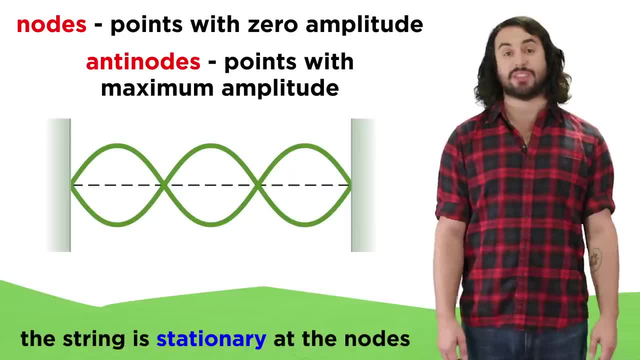 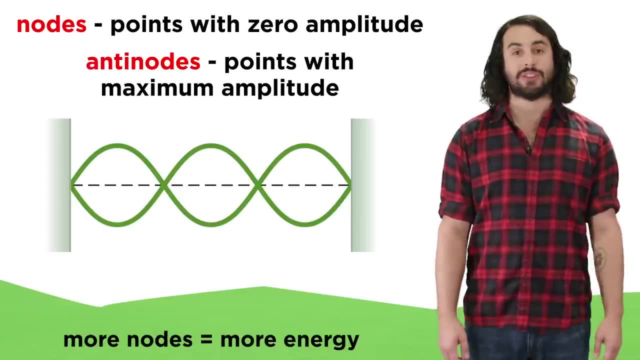 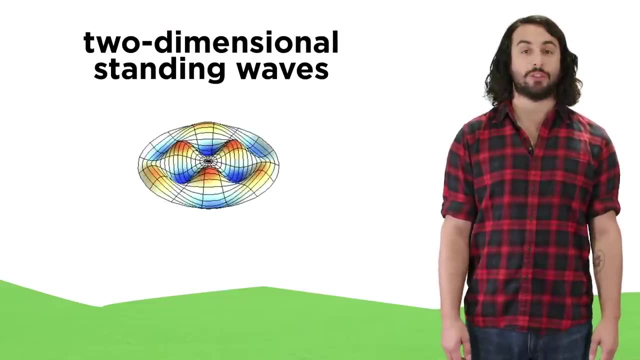 The string will be completely stationary at the nodes and the other sections. if vibrating rapidly enough, will appear to the human eye to create loops. And more nodes means more energy. Two-dimensional standing waves also exist which manifest on a flat two-dimensional surface. 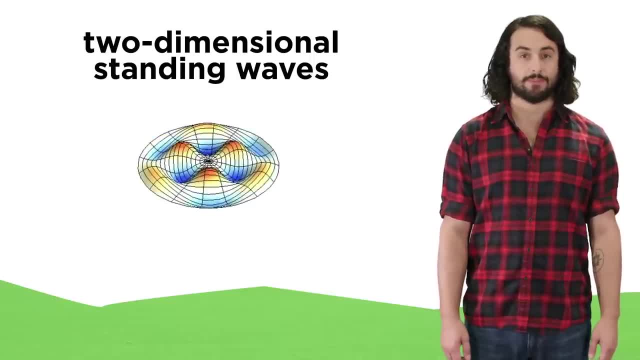 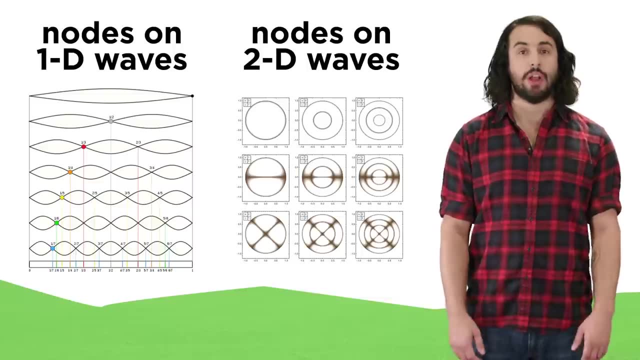 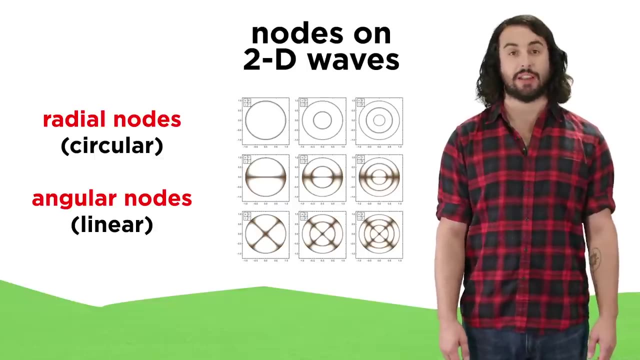 like a drum head rather than a one-dimensional string. On a one-dimensional string, the nodes are points, But on a two-dimensional surface the nodes are lines and curves. These can be radial nodes, which are circles of a particular radius, and angular nodes. 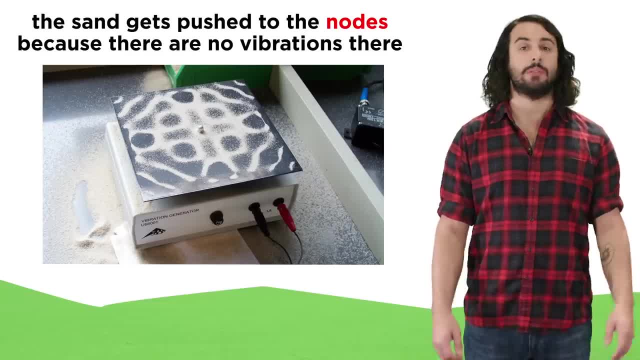 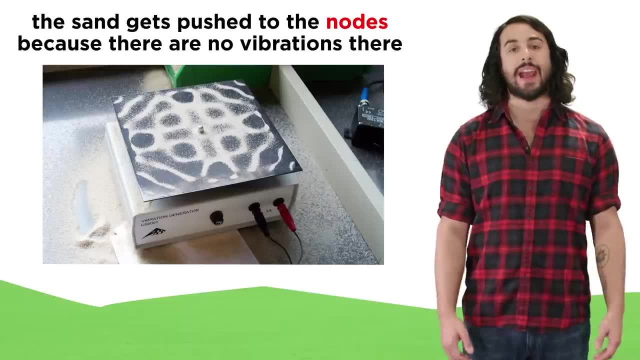 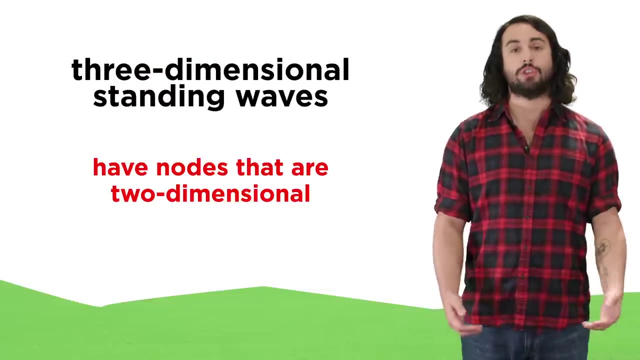 which are lines at particular angles. These nodes can be visualized if we place sand on a vibrating surface. The sand gets pushed over to the nodes by the vibrations and this helps us visualize the two-dimensional standing wave. A three-dimensional standing wave would have two-dimensional planes as nodes, but we will. 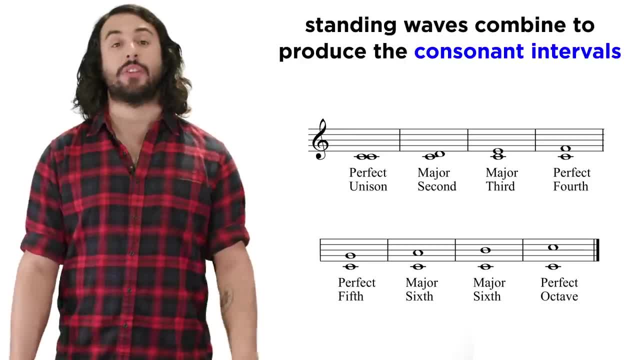 have to use our imaginations for that. One interesting thing about standing waves is that they combine to produce all of the consonant intervals in music that describe the two-dimensional waves, So they can be visualized as two-dimensional waves, but they also have to be visualized. 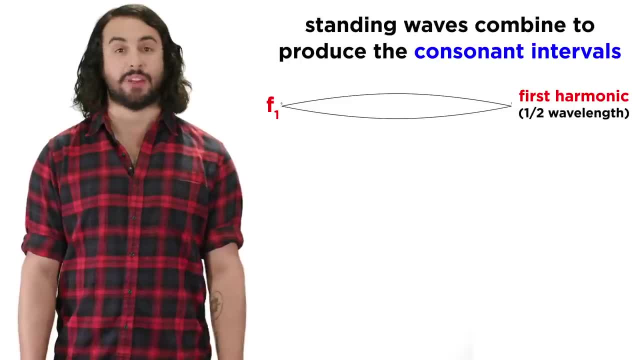 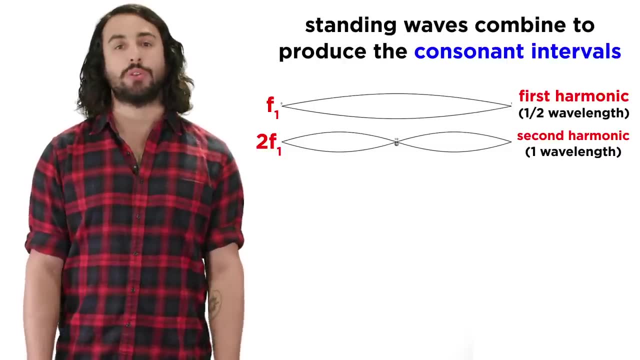 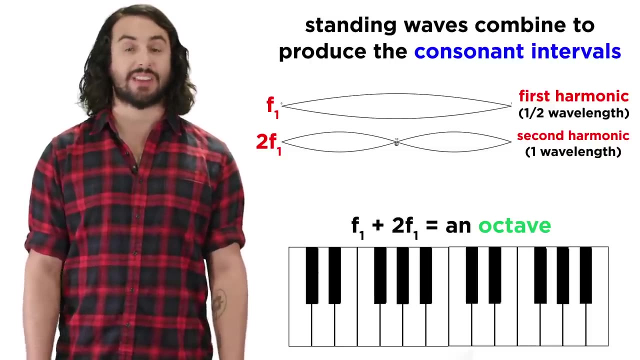 sound good to our ears. If we consider this half wavelength to be the first harmonic with a frequency of F1,, then doubling this frequency to 2F1 will produce a standing wave with one full wavelength and will give us the second harmonic, which in music would be perceived as an octave. 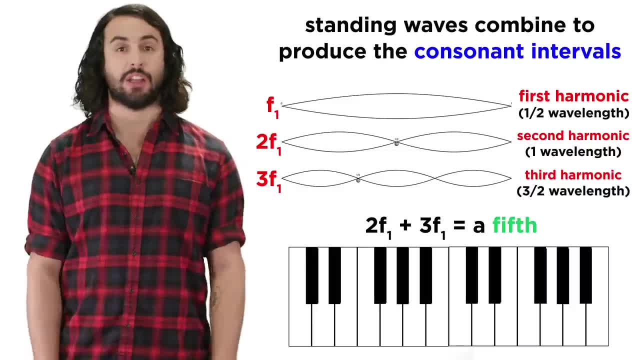 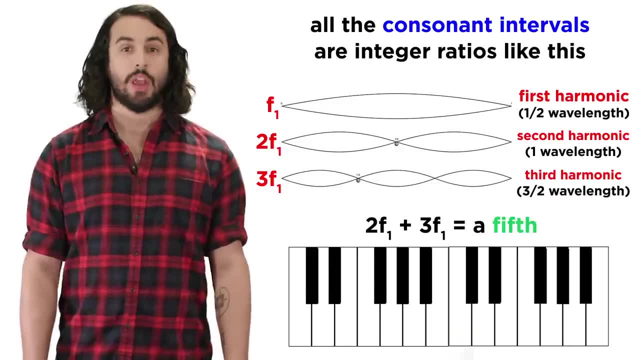 Tripling the original frequency to 3F1 will give us the third harmonic, which in music is called a fifth. This will continue to give the rest of the consonant intervals. So the reason that certain combinations of notes sound pleasant is no random matter. 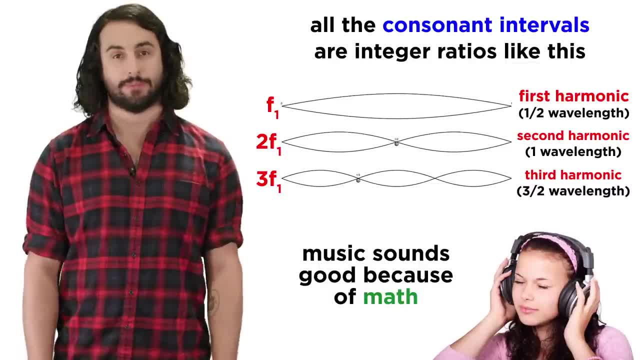 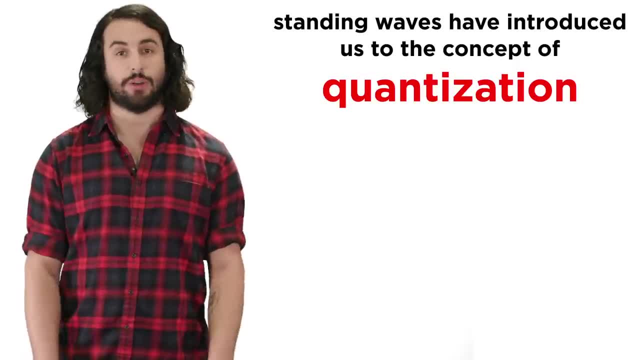 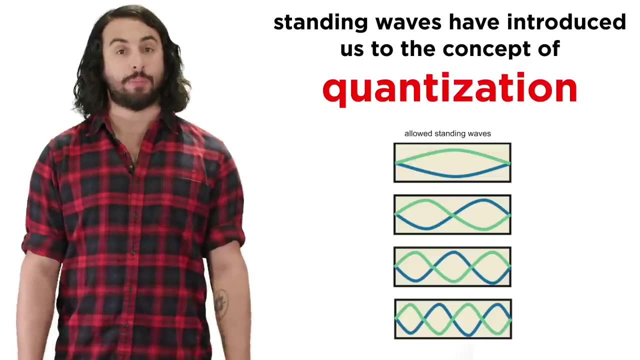 it is rooted in the harmonics of standing waves. This concept of standing waves also represents our first encounter with quantization, given that each harmonic has an integer number of half wavelengths, and quantization will be a very important concept in the modern physics course.